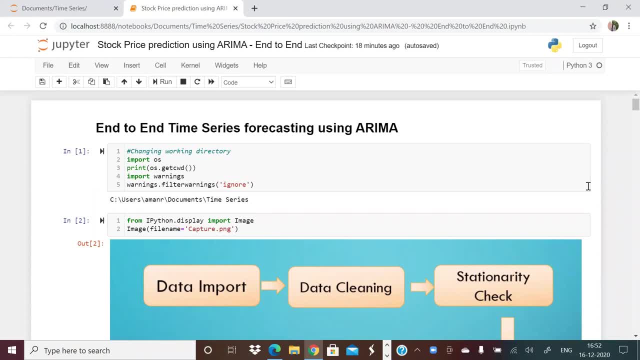 Hey guys, welcome to unfold data science. This is Aman here and I am a data scientist, As you can see on your screen. guys, today I am going to show you an end to end implementation of time series, basically using the ARIMA method. So most of you would be heard, would have heard. 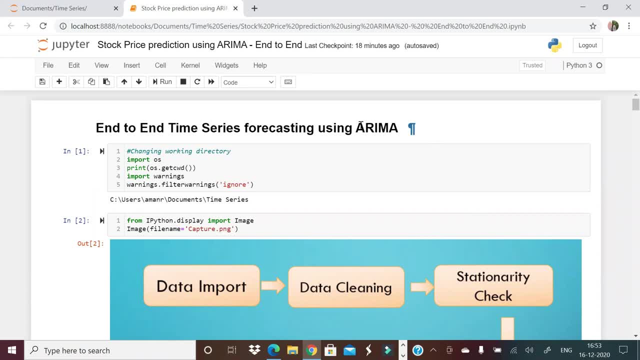 about the method ARIMA, which stands for auto regression, integrated moving average or auto regressive integrated moving average. right, So there are three components of ARIMA. one is AR, next is IE and this is AMA. AR stands for auto regression, MA for moving average and I4 difference in term. I have already explained AR and MA in my in the same playlist in my. 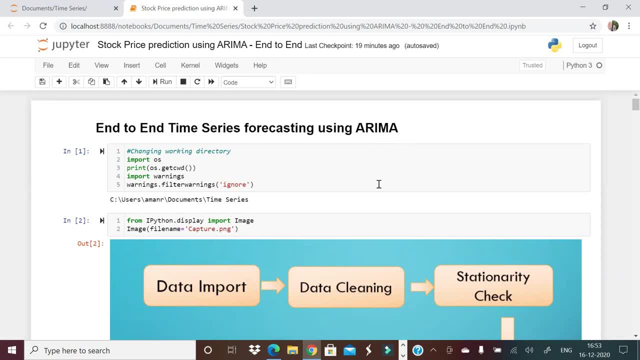 previous videos. I am giving the link. you can watch those videos as well, But in this video we will see an end to end implementation of ARIMA as a model. Okay, So what I am doing here is I am just setting my working direct tri plays here. as you can see, this image was. 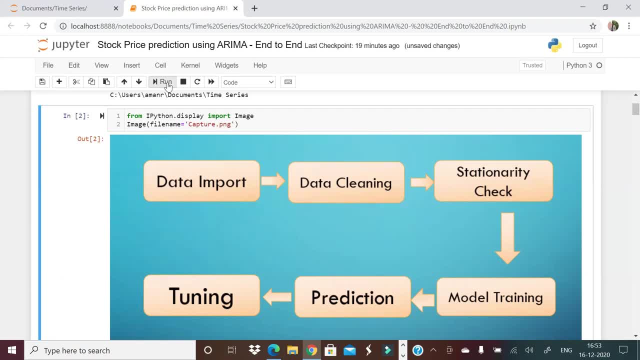 used in my seen here last video as well. I'm importing the data cleaning, doing some stationarity check, I will tune, I will train the model- Arima model- Then I will do some prediction and then I will tune the model. We will do all this step by step. This video might get a little longer. 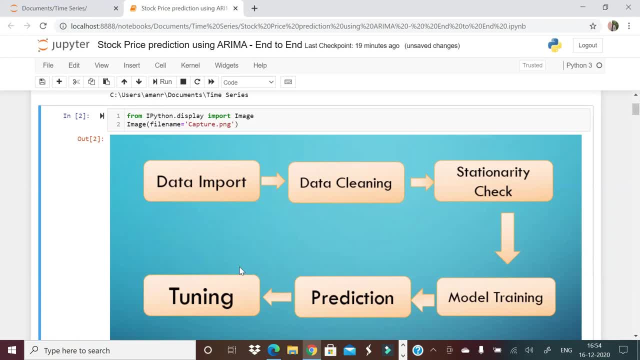 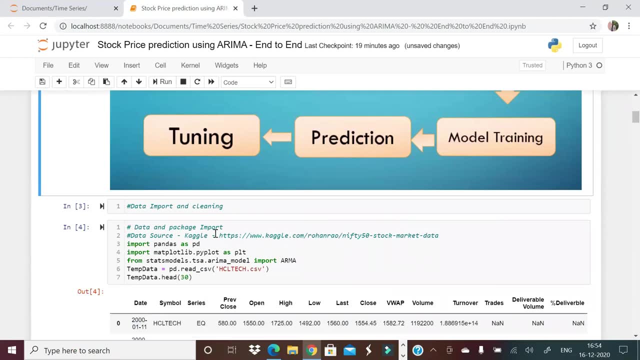 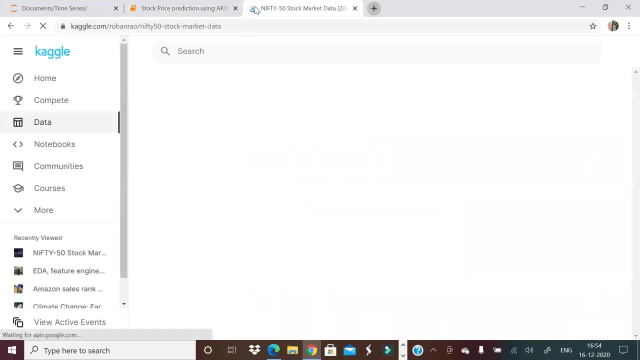 but I request you to watch till end so that you get a overall understanding of how to fit a time series model. So first thing is guys importing data. Okay, So where from I have taken data? I have taken data from this place. Okay, so a credit to caggle and in caggle, credit to Mr. 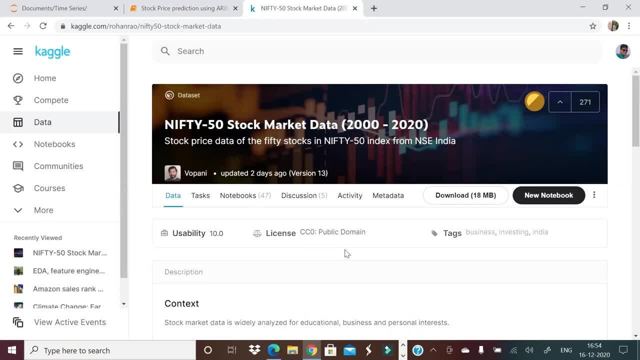 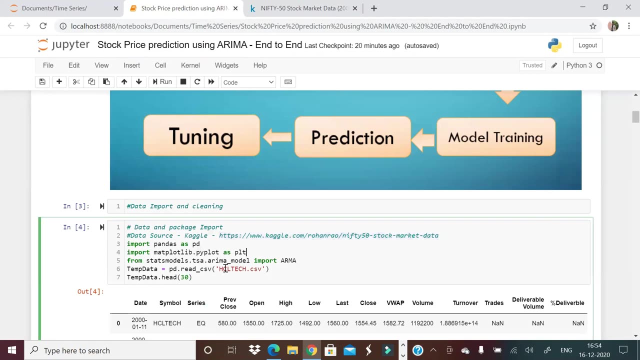 Bopani, who has uploaded this data. So this data gives you stock market data, basically the nifty data for different different stocks. Okay, so you can download the data from here. I'll give you the link and I can give you the data as well. Okay, In this data I am taking one particular company. 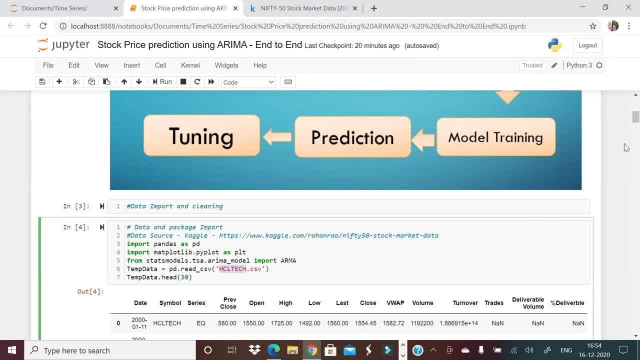 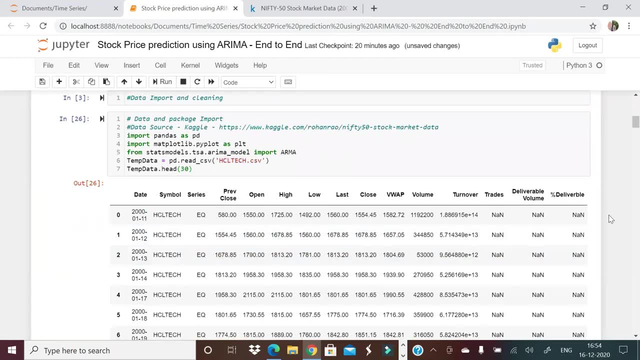 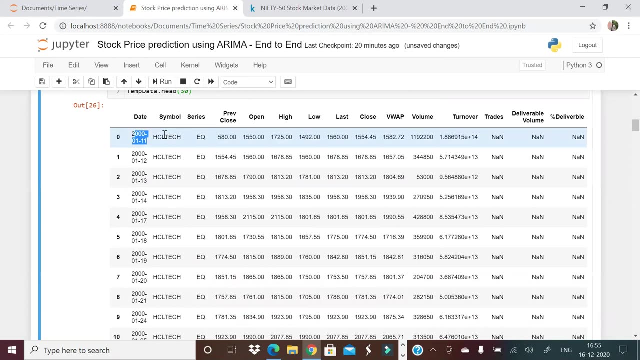 at CL Tech. Okay, so it's CL is a software company. at cltechcom tech data i'm taking and i'm just printing the first 30 records of hcl tech data. so, as you can see, guys, the on from the year 2000. okay, symbol: hcl tech. hcl tech is the name of the company. 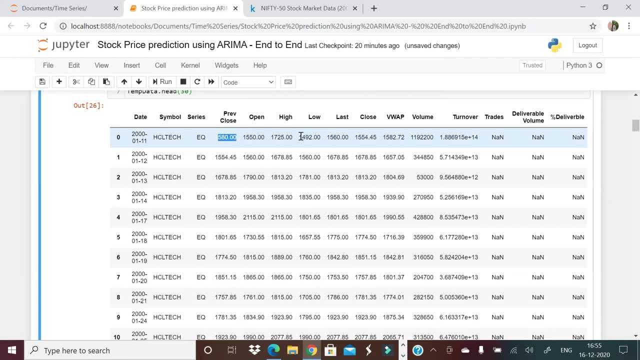 previous close. this is the stock market price: open, high, low, last. all these things right. what was the previous close, what was the day high, what was the day low? all this information of this stock price right. so we will be using this previous close column as our main column for on what? 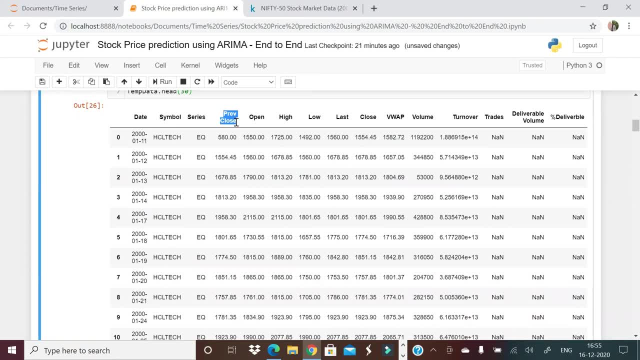 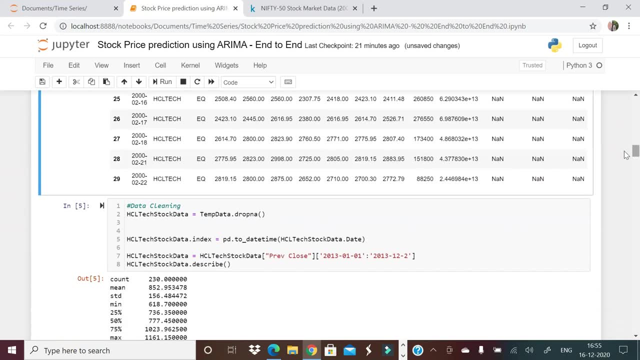 target or on what number this stock price will close for that particular day. okay, so going forward, i will use this column only so what i am doing here is i'm dropping all the na columns so that our analysis is not disturbed. i have many records, so i can drop some of these ns. 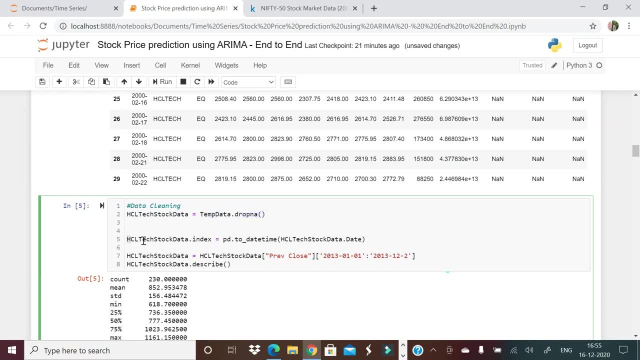 right next thing, very important thing, guys: you have to necessarily make a index column in any of your time series analysis. so, as you can see, there is one column called date, this date column. i am making it as the index column for this analysis. okay, so i'm. 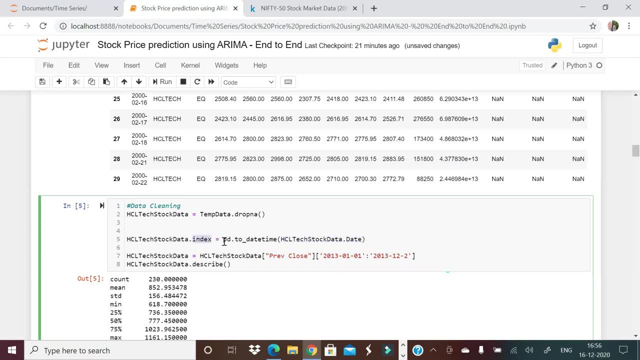 saying hcl tech stock data dot index is equal to pd dot date time- this date. so it will take this date as my date column. okay, now i am taking as i told you, i'll be using only one column and i'm taking the data from 2013 as a. 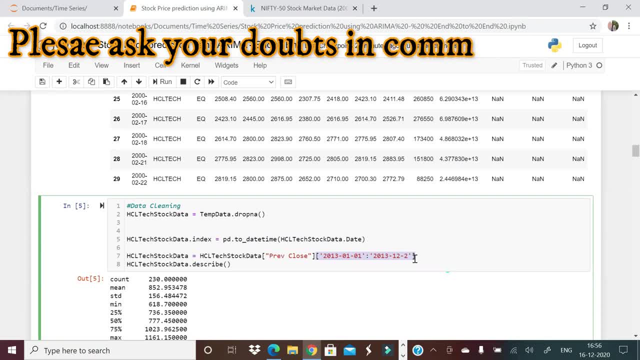 date column. okay, now i'm taking, as i told you, i'll be using only one column and i'm taking the data from 2013 as a year. okay, 2013, from january to december, as you can see here right now, if you come down, guys. so i'm. 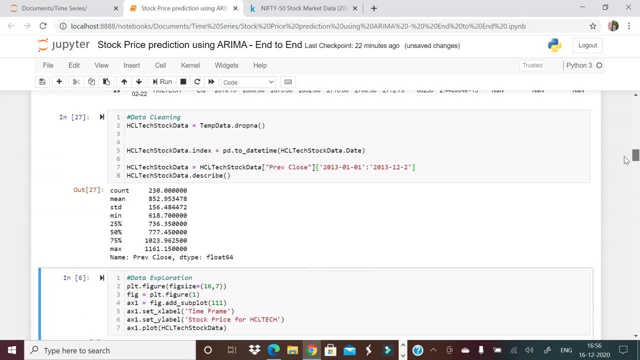 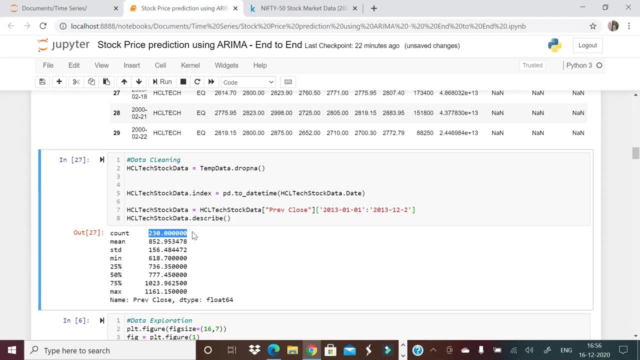 just printing a describe of my data- so nearly one year of data. you will see some 230 entries. the reason for that is on saturday and sunday, stock market holiday is there and some more holidays, right. so nearly 230 entries. the mean is 852 and other percentiles you can see here. now let us plot. 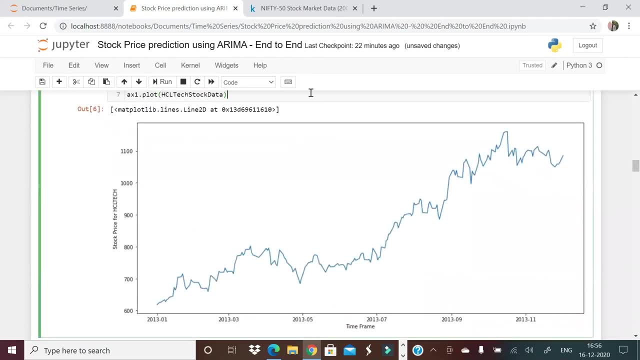 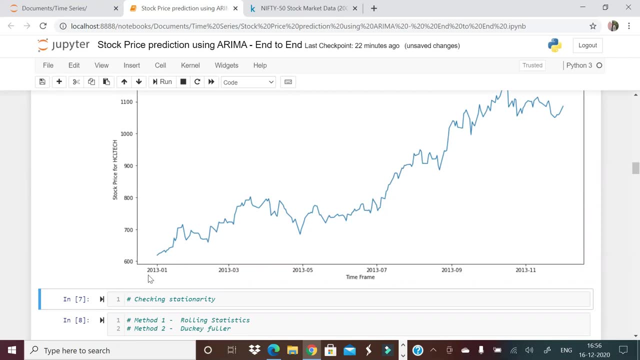 this data and see how it is going to work. so let us plot this data and see how it is going to work. is looking like? okay? so this is the plot of the hcl tech stock data guys for 2013, entire year. okay, this is the first month 2013. this is 11th month and then the 12th month. okay, now, as you can see, i have 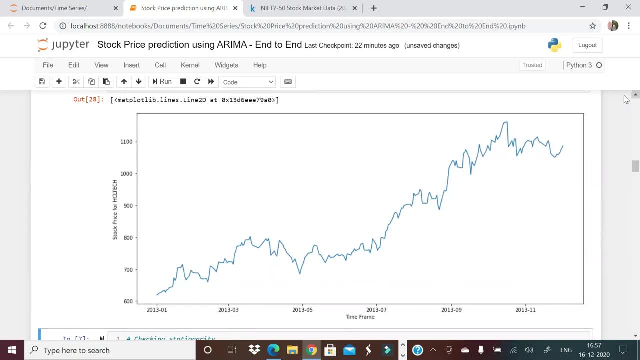 knowingly taken this data, the reason being it is showing some kind of uh, i can say it's not an easy time series. okay, so there is no clear-cut trend. sometime it goes up, sometimes it comes down, again it comes down. sometimes it goes up, sometimes it goes down. sometimes it goes down, sometimes it goes. 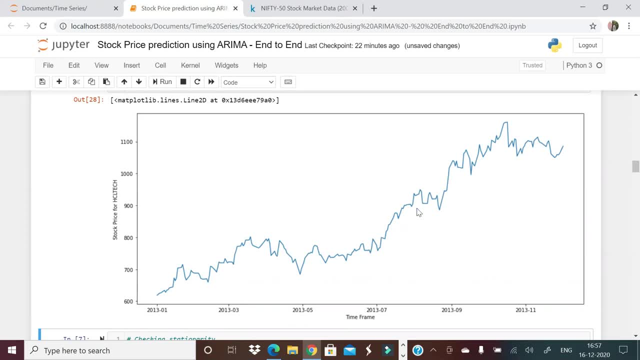 down, goes up, comes down, so there is no fixed. uh, what you say, seasonality component or trend is there. of what trend is there? but seasonal components we cannot see clearly in this image. okay, so how do we see the next thing about these time series? the very first thing is, we should know. 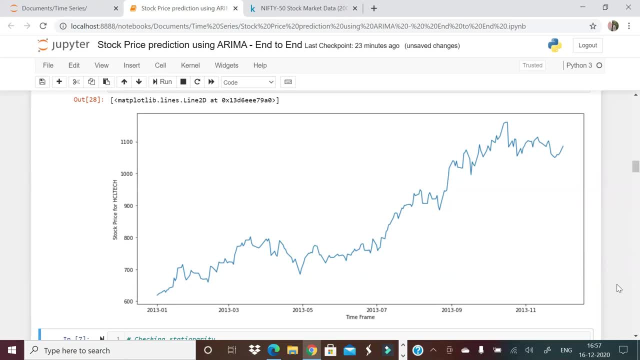 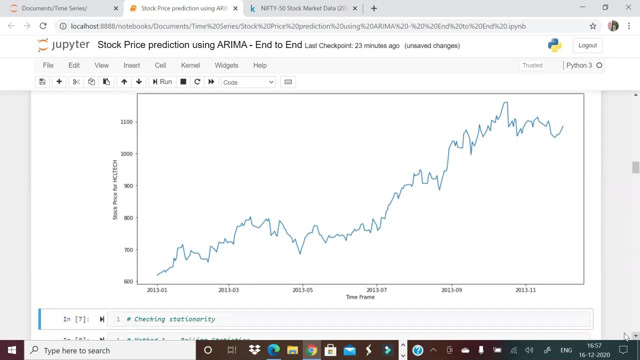 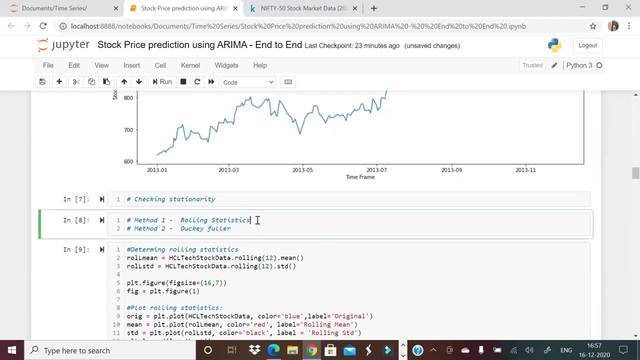 whether this is an stationary time series. how do you see whether the time series is stationary or not? again, i have created a video on that. you can watch that video. to keep it simple, you can use two methods. one is using rolling statistics, which means rolling mean and standard deviation. next is using 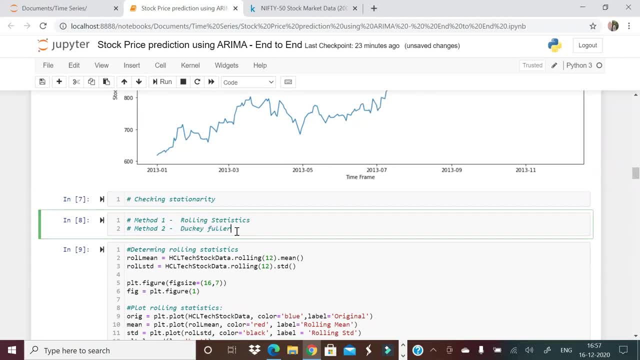 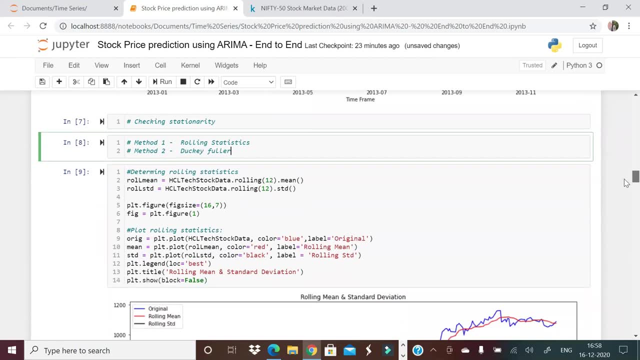 ducky fuller test both these methods i have shown you in this video. the link is right here. you must watch this video as well. okay, and then what i'm trying to do here is i'm trying to create some rolling statistics. if you see, rolling mean is equal to hcl stock data dot. rolling 12 mean. 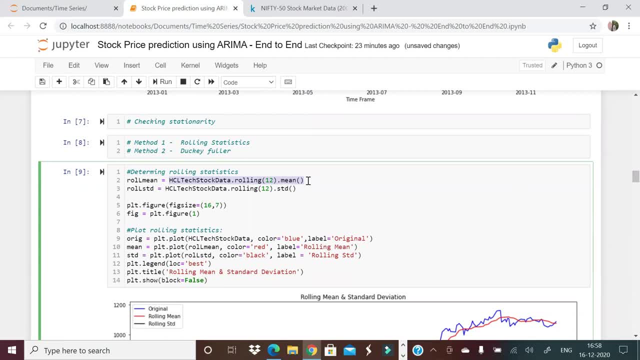 which means i'm taking a rolling mean of last. i'm taking a rolling mean of 12 entries. okay, similarly rolling stat standard deviation of 12 entries. and don't worry about these plot things, guys. this is just about plotting these two numbers. okay, now i'm plotting the original series with. 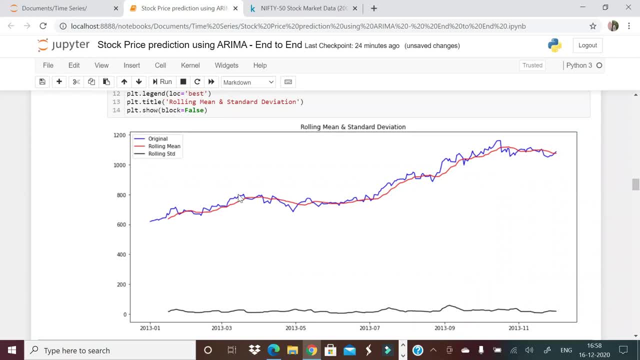 the rolling. okay, so original is blue in color, rolling mean is red in color and rolling standard deviation is black in color. so, as you can see, rolling standard deviation is more or less constant over the time. okay, so what is the uh prerequisite for a standard deviation series to called stationary mean should be constant over a time and standard deviation. 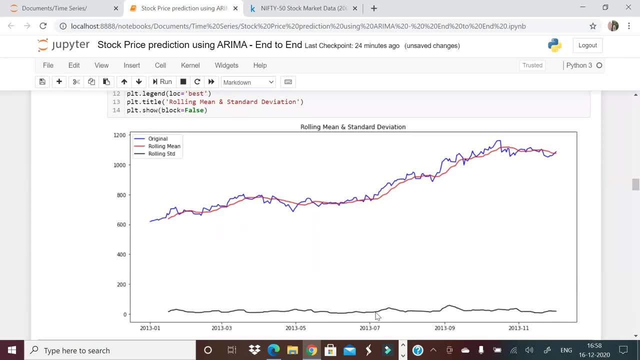 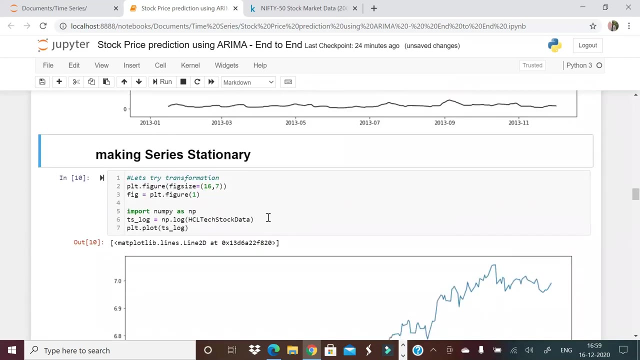 should be constant. over a time now we can see rolling standard deviation is kind of constant, but rolling mean is not constant, which definitely means that this series is not a stationary series. right now, coming back to how to make this series stationary: plt dot. plot figure size is equal to 16. 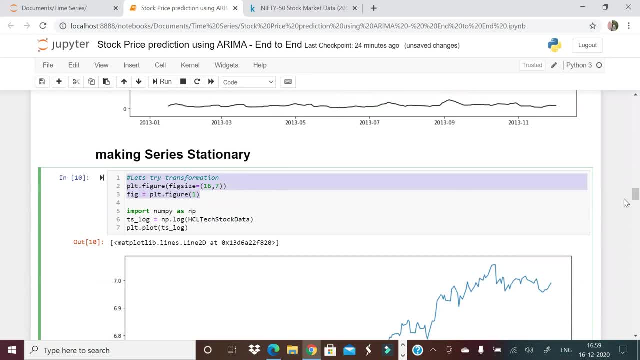 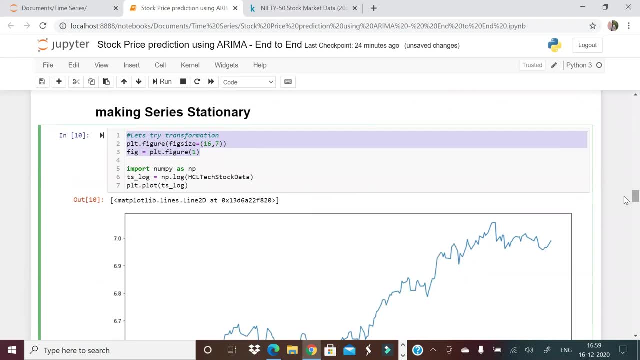 7. figure size is equal to. so i'm just giving the figure size. and then the first thing we can do is to make series stationary. is we can take a log transformation of this series or we can take many transformations. so here i'm taking a log transformation. 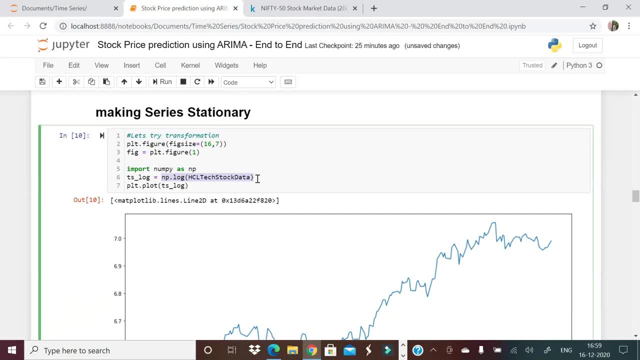 you can take a square root transformation, cube transformation, many kind of transformation. we don't know what transformation will make our series stationary. okay, so i'm just trying with log transformation. np dot log will do the log transformation of my series and i'm plotting that. when i plot that, 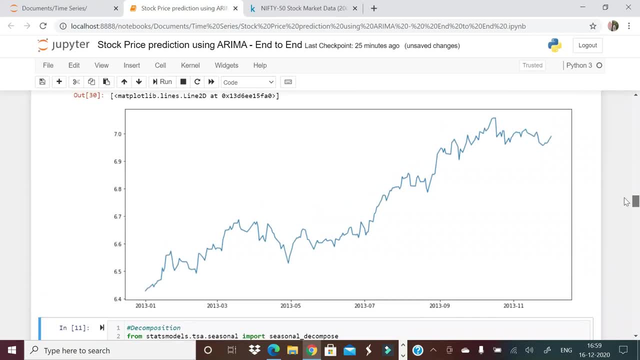 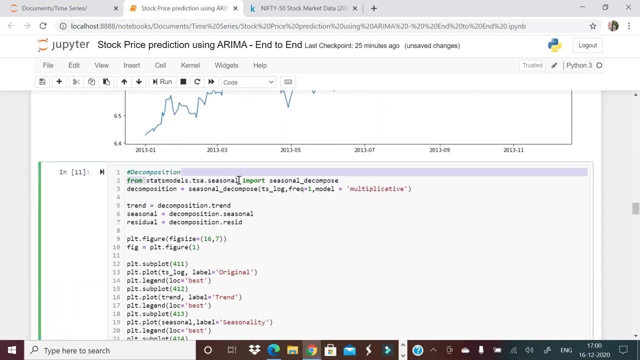 this time series is not becoming stationary. as you can see, stationary time series will not show a trend like this. right to to double sure that this time series is not stationary, we will just decompose it into seasonal components. okay, how to do that? from stats model tsa or. 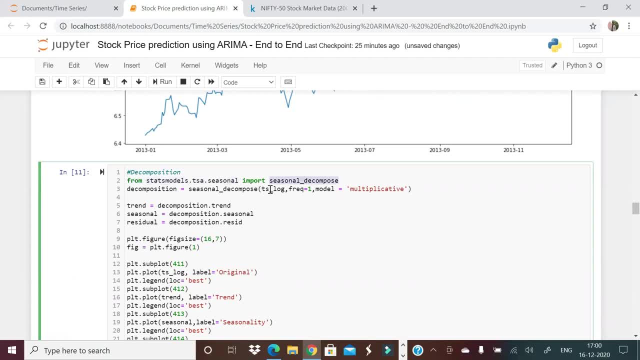 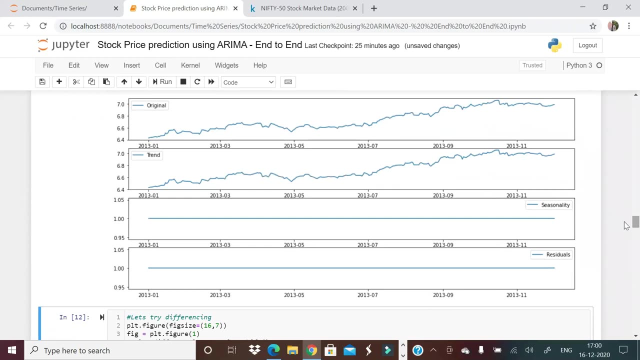 seasonal import. seasonal decompose. decomposition is equal to ts log- and what this will do is it will give you the different components of your time series, whether it is a seasonal trend, okay. so if you see this chart here that that particular time series has been broken into four, 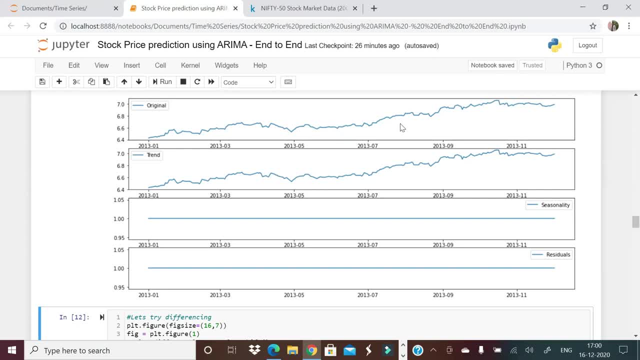 components. the first one is the original uh series. second one is the trend component of that particular series. third one is the seasonality component of that particular series. and fourth one is the residual component of that particular series. so it is very evident from here that trend component is contributing more to the original time series. 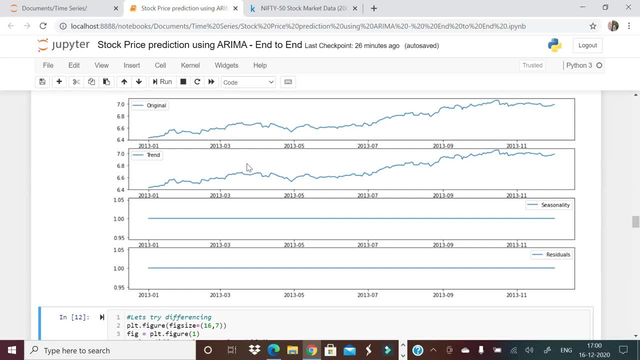 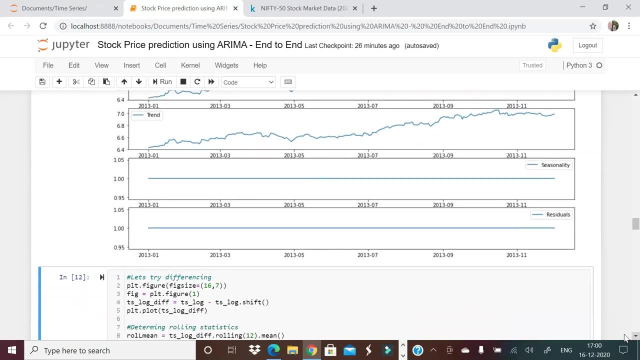 right now. we know series is not stationary, even after log transformation as well, so i will do something else. what is that something else? so i will create a difference to time series. what is difference to time series? i will shift the time series by 1 and subtract from the original time. 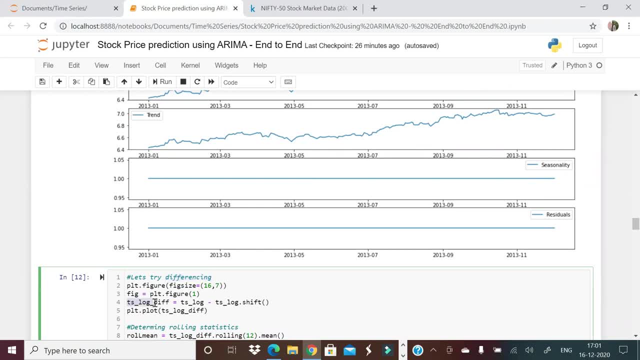 series. that is what i am doing here, guys. ts log difference means the logged time series, and then i get the difference is equal to 2 right to TS log minus TS log shift 1. So I will get a differenced time series as a result. 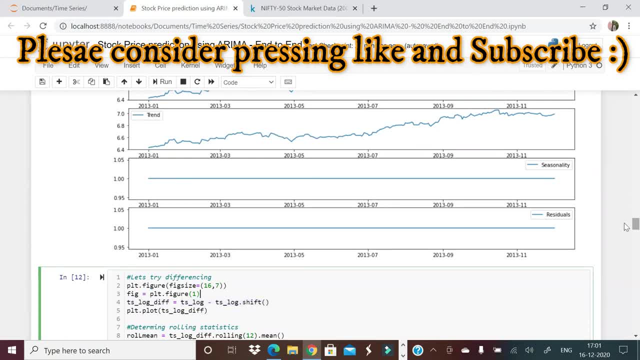 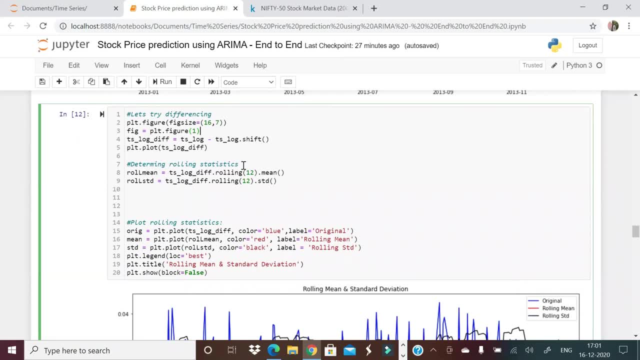 of this, and then I expect this differenced time series to be stationary, at least. Okay, So same way, I am plotting the rolling mean and rolling standard deviation on this time series. now, Okay, To check whether this is a stationary or not. When I do that, guys, you 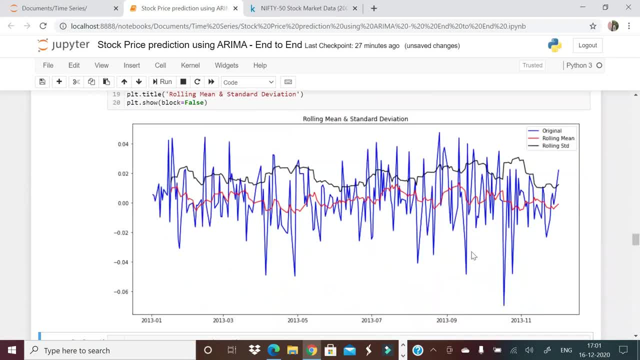 can see. the blue one is my differenced time series. Okay, The black one is my rolling standard deviation and the red one is my rolling mean. Now you can see there is no upward pattern in the mean and there is no upward pattern in the standard deviation. So by the definition, 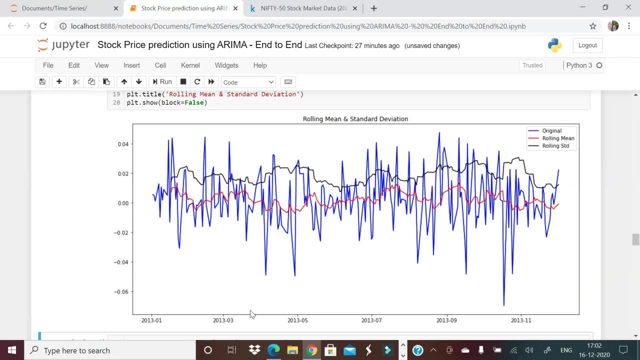 of stationarity. if I take mean between these two points, and if I take mean between these two points, then there will not be too much of difference between these. So I assume this time series will be a stationary time series. All this hard work of taking the log. 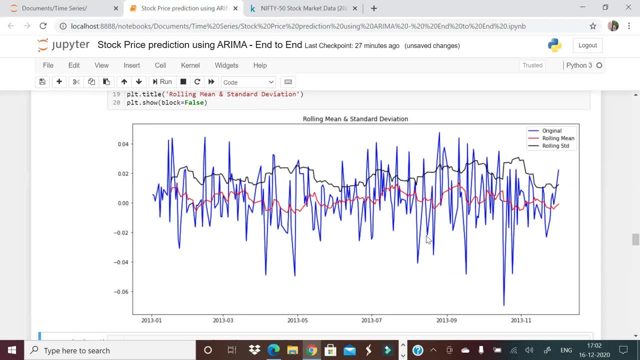 and taking the difference and seeing the mean, seeing the standard deviation is because we want series to be stationary, otherwise our model will not fit well on the series. Okay, And also we have to remember what all transformations we have done, For example here we have done. 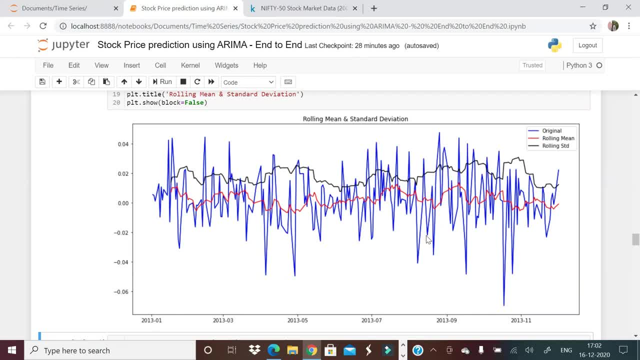 log. and here we have done differencing. Just remember these two. Okay, Now this time series looks looks good, guys, Good in the sense looks stationary. If you want to cross validate, you can do a Dickey Fuller test as well. Okay, Moving. 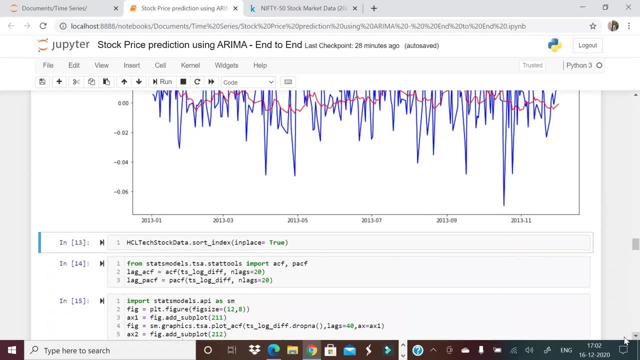 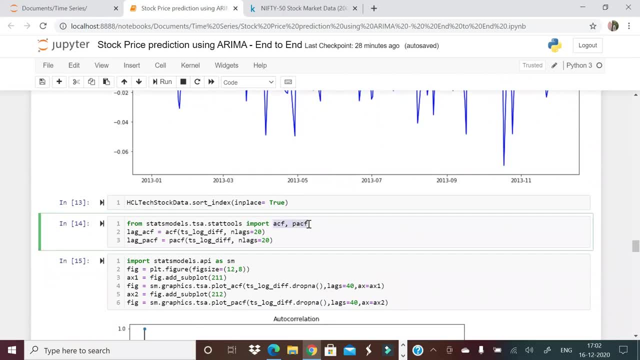 on to the next steps. guys, Now we have a time series in hand. Let us try running ACF and PACF. Now, what are these two things? I have explained this also in one of my video in time series playlist. These are important to determine what will be the order of your 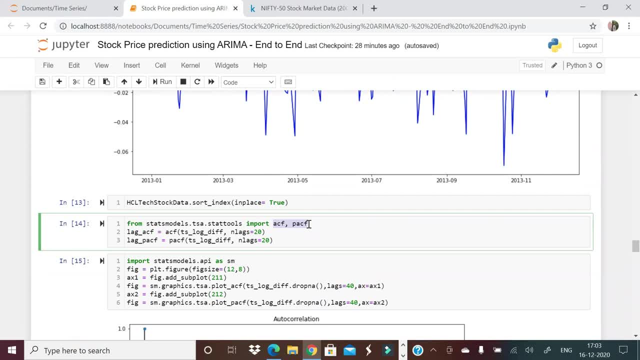 AR component and MA component in the Arima model, Okay, One is called autocorrecting, Okay, And the other one is called autogest, Okay, So the auto-correcting is called autogest. So the auto-correcting is called autogest, Okay. So we have the auto-correcting which we are. 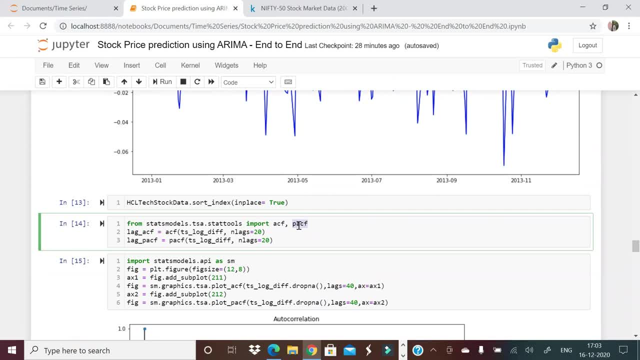 correlation plot. second is called partial autocorrelation plot. okay, watch the video on these topics as well. link I am providing. okay, now what I am doing is I am plotting ACF chart and PACF chart for that differenced time series. okay, let me do that. this is how your 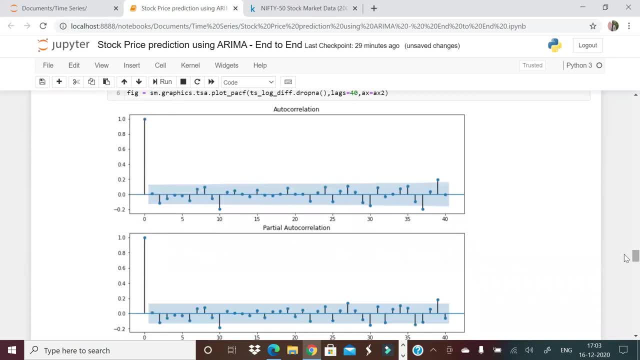 PACF and ACF looks like now. how do you determine from: first one is autocorrelation, second one is partial autocorrelation. the important thing to understand here, guys, is whenever you are running a arima model, you do not know what order of AR and MA or I will be good for your model, okay, so 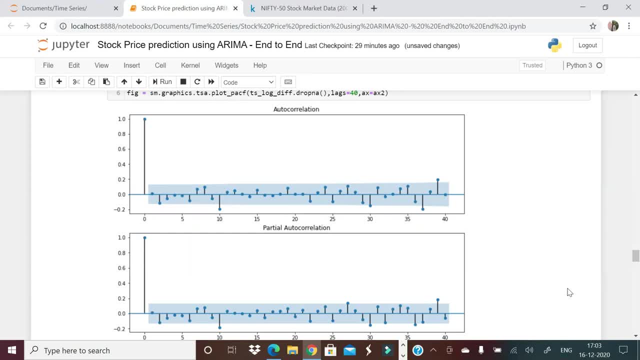 these charts help you understand in that now, the thumb rule here is: whatever the highlighted part you see here, these are called confidence intervals. okay, and the first line that crosses this chart, the first line that crosses this chart, is the line of your order, whatever you want. now, here you can see. I am just considering. 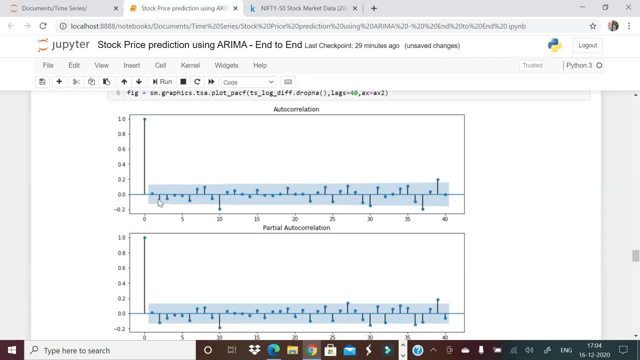 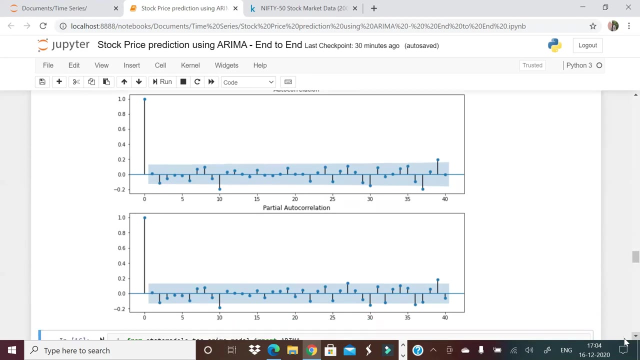 line number two. so this is point number zero, point number one and point number two. here point number two is not crossing the interval, but it is just touching the tip. okay, so I will consider order of AR as two. okay, from autocorrelation. order of MA. also, I will consider two from partial. 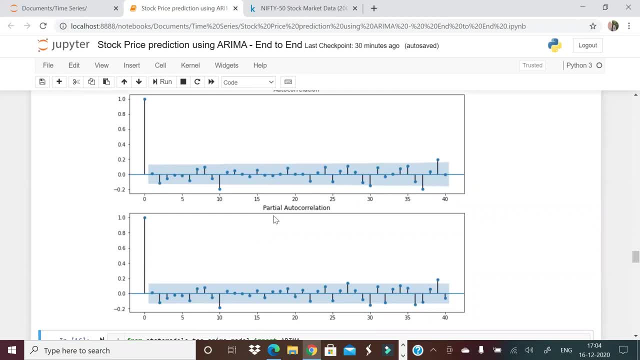 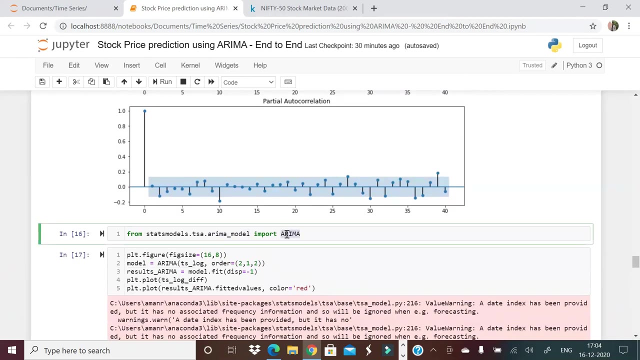 autocorrelation. okay, I do not know whether that is the best fit, but to start with, let us go with two zero. two as PDQ, okay, and D- I am starting with zero, let us see what happens. okay, so what I am doing here, from stats model arima, model, import arima, arima- give your time series, okay, and then order will be two. one. 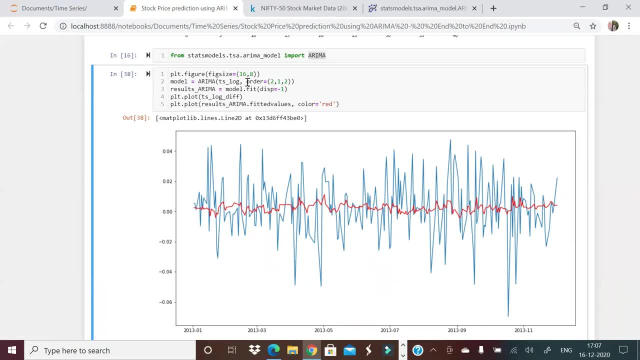 and two. okay, so here I am starting with order two: one, two, as you can see right, and then when I run these guys, you will see that this red one is the fitted values, which means I am predicting for that model, and this other one, the light green one, is the actual values. so this is how the time series model is fitting on the data. 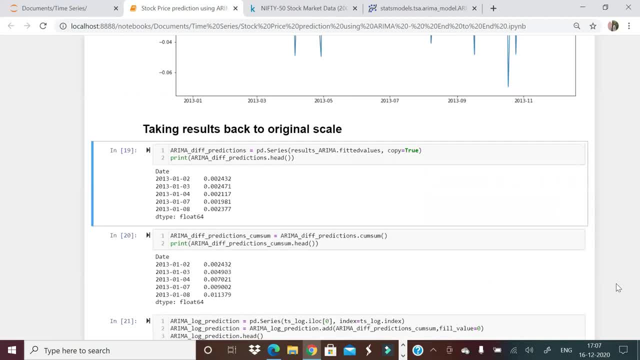 now what we need to do is we need to. we have done many transformations right, so we need to taking result back to the original scale. so I told you we we did nplog, which means we did the log transformation. we did some bit of differencing right. 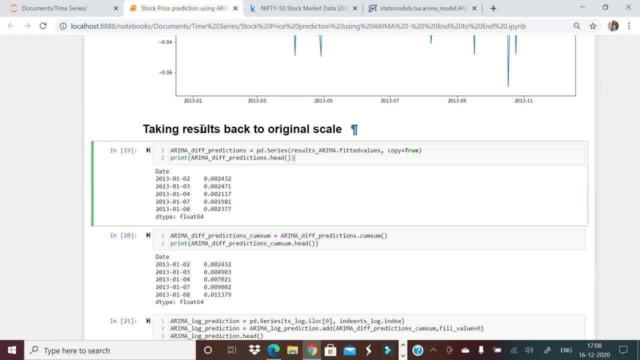 so in the first step, what we are doing is we are just taking the fitted values in a in a series. in the second step, what we are doing is we are taking the cumulative sum, the reason being we differenced the time series, okay. and in the third one, what we will do is we will take the 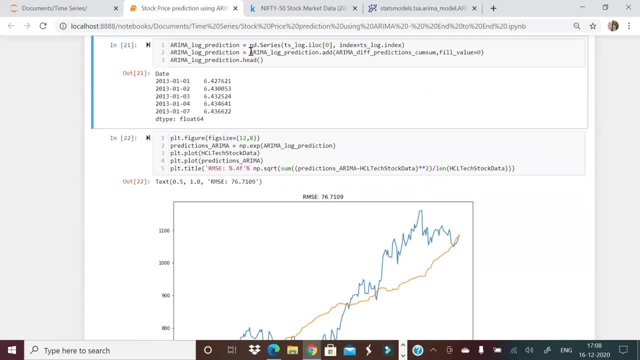 np dot. as you can see, there is one step before this. what we are doing is we are taking log prediction and we are adding. this addition is to compensate for that differencing. okay, we did that differencing. if you see one one values, you will understand what is happening, right. and then in 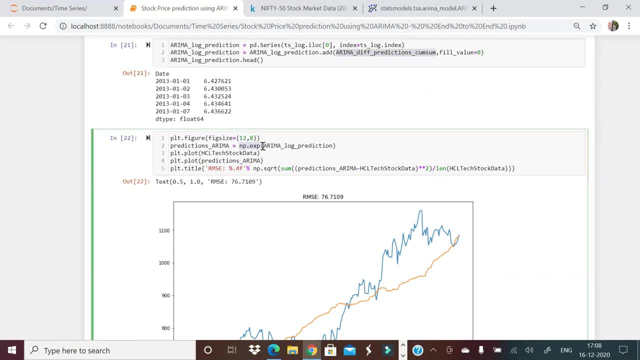 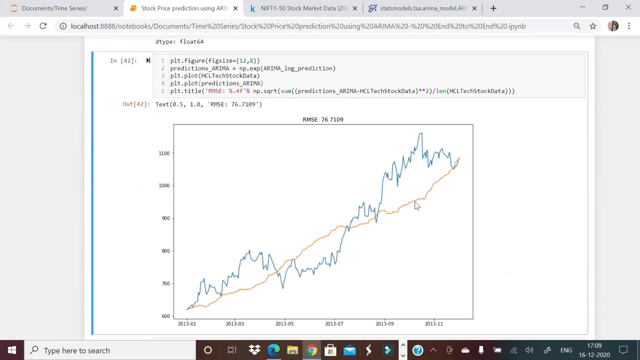 the last step. if you see we are doing npexponential, so what is the reverse of log guys, exponential, right? so since we had done log, so here we are doing exponential, so npexponential, arima log prediction. and then when I run this you will see that this, this pink one, this light pink one- sorry, the orange one- 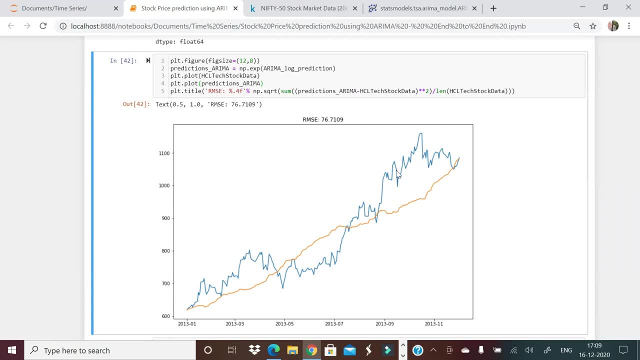 is your predicted value and the light blue one is your actual values here. okay, now there are many things about this time series which we need to understand. one is: this time series is very well capturing the trend component, but the time series is not capturing some of these unexpected ups and 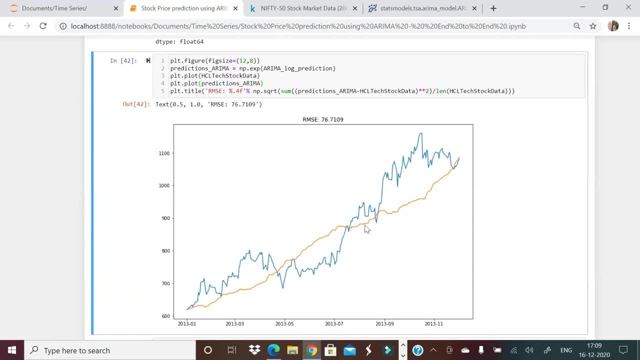 downs. there are some minor ups and downs in the time series, but volume of those is not as par with the actual time series. okay, and that is where we are getting some RMSE values here. how to improve that now? if you remember, we started from pdq as 212. okay, we do not know if 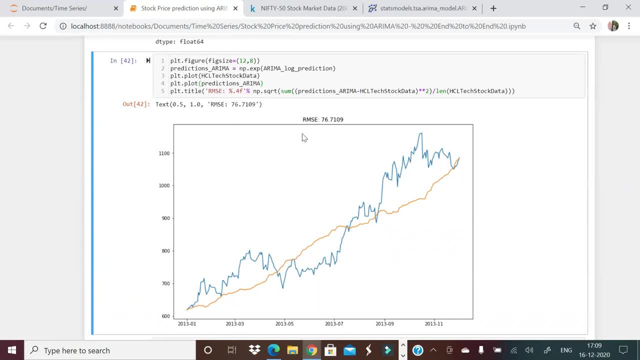 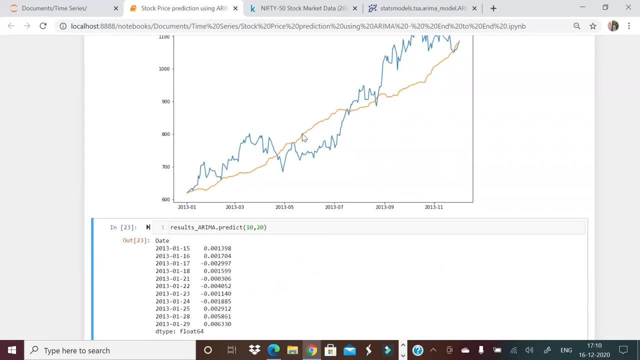 some other pdq will give a better result for the same time series. there is another way in which we can do it. the way is known as auto arima. before that you can predict using that same model result: arima is a dot: predict and for whatever, to whatever entry you want to predict, you can give in the for. 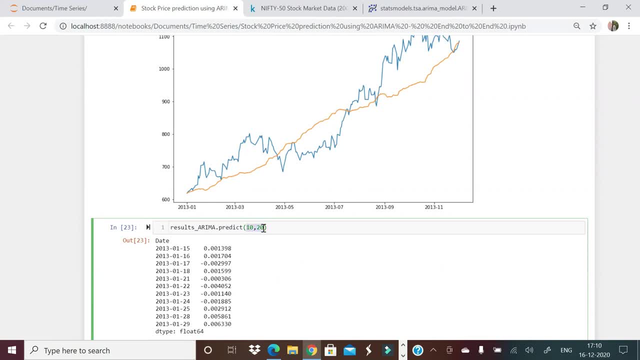 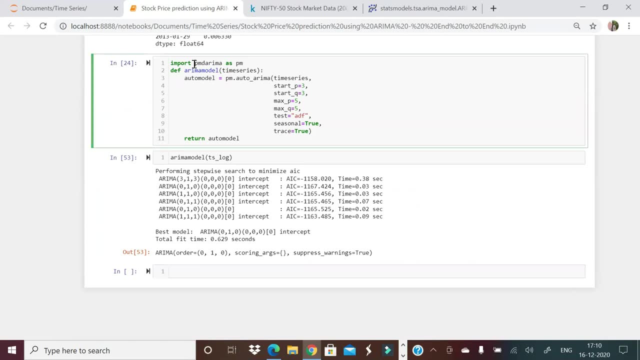 so, for index number 10 to inch number 20, I want to predict, and these are the predictions. Okay, I was talking about auto arima as well, So auto arima comes from a package called PMD arima. You can take your auto arima. 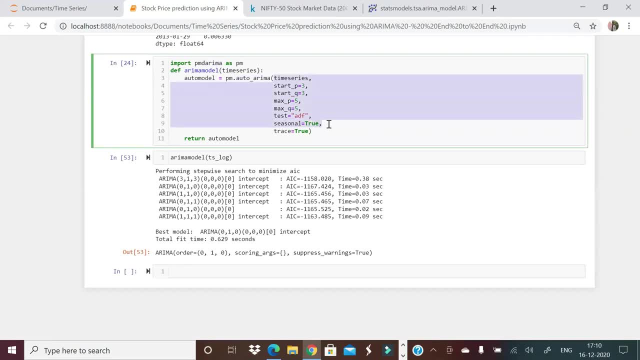 you can give your different values of PDQ and run that in a loop. Okay, what will happen is it will give you the best PDQ values for your model. Now, when I ran that auto arima for this model, I got the best PDQ as 010.. When I plugged in 010 in my model, I was not able to get a better. 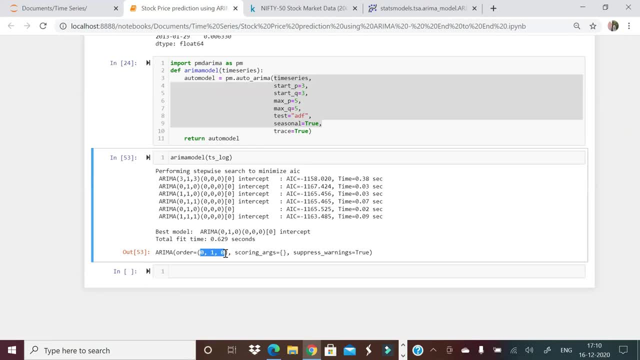 performance. So what I'm suspecting is there could be a better way of making this time series stationary and there could be a better way of doing the transformations. So I leave it to you. you take the data, you see this notebook also and you try to implement this time series in your own. 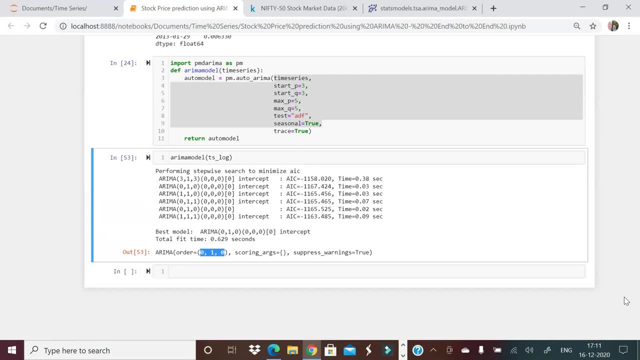 local environment and try to see what transformations help you, What, what other things you can do so that your time series performance can be better. Okay, But all in all, this was an implementation of arima, all the steps involved, just to reiterate you. 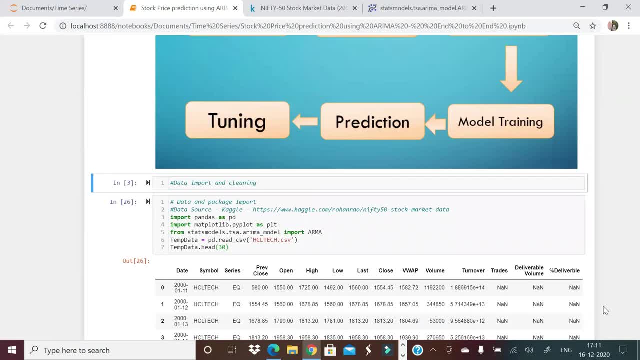 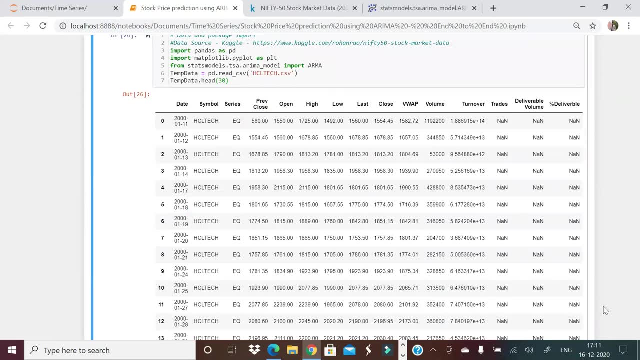 import the data. you clean the unnecessary stuff, you ensure data is stationary and then you take it to the model And then you decide and which which is the optimal PDQ for your model. you run the time series. if there is performance can be improved, you improve with auto arima or 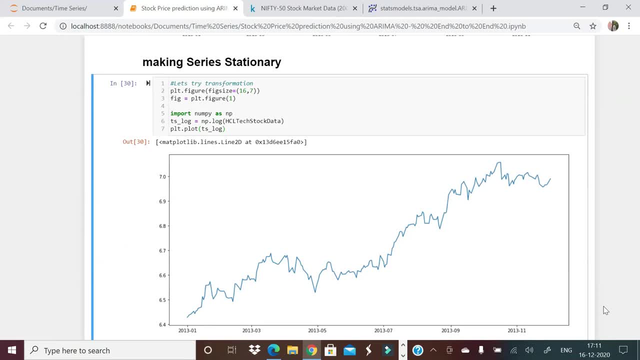 you run the time series. if there is performance can be improved, you improve with auto, arima or other differencing methods or transformation methods, right? So this is all in all that I wanted to show you in this video. guys, Let me know what doubt, what questions you have. 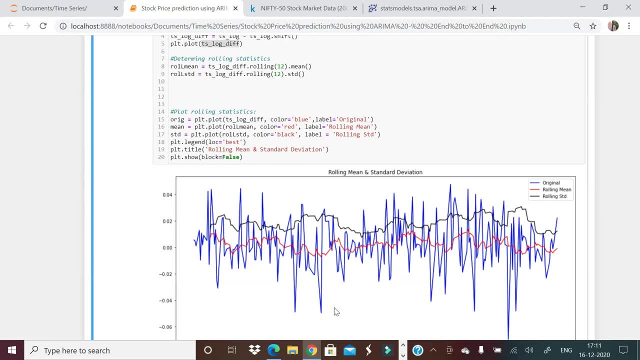 I'll see you all in the next video. Till then, all of you, stay safe and take care. 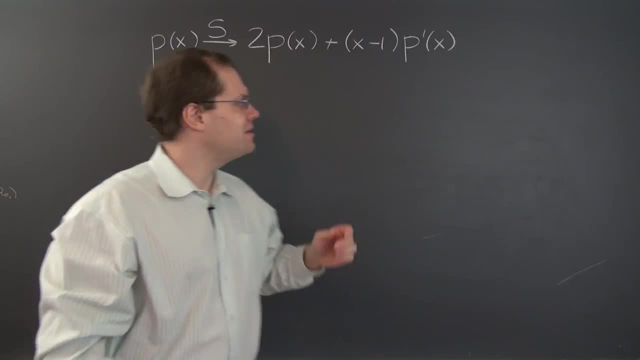 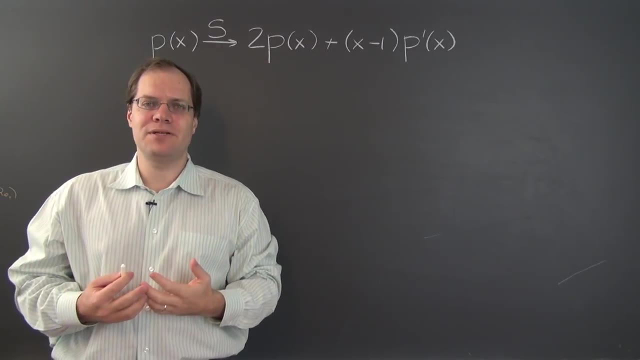 Next, let's consider a polynomial transformation. Here I have a linear transformation denoted by the letter S, because it is, after all, a very silly transformation with absolutely no applications, but it's a linear transformation nonetheless, so it makes for a perfectly good example. 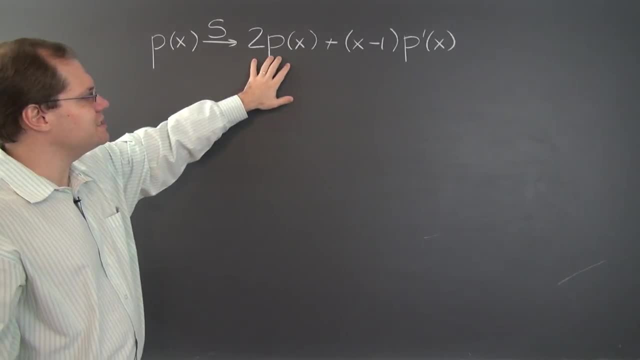 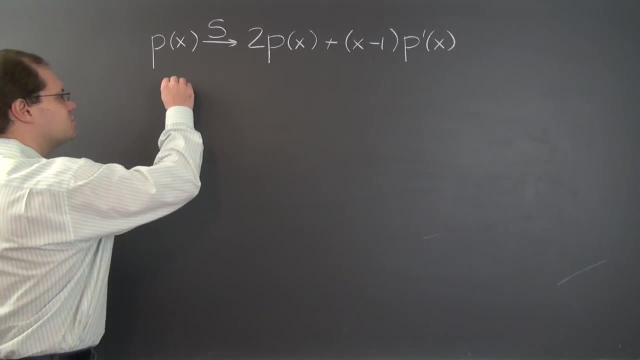 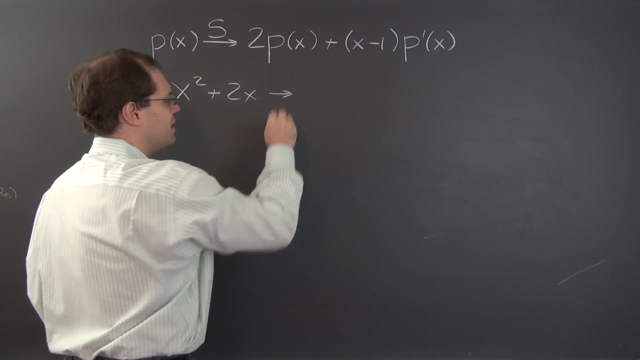 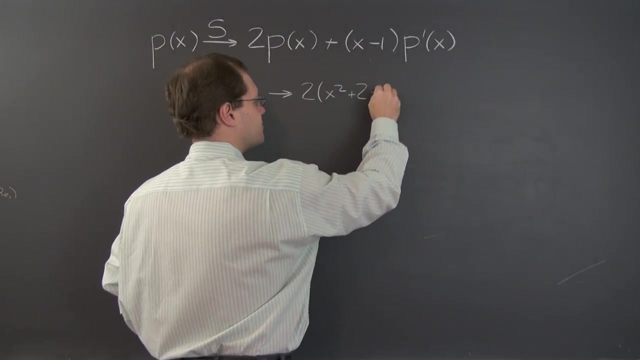 So any polynomial is transformed to twice itself, plus x minus 1 times its derivative. So totally silly transformation. but just to get an idea of what it does, let's apply it to x squared plus 2x. Okay, and x squared plus 2x becomes twice itself. so 2x squared plus 2x plus x minus 1 times its derivative. 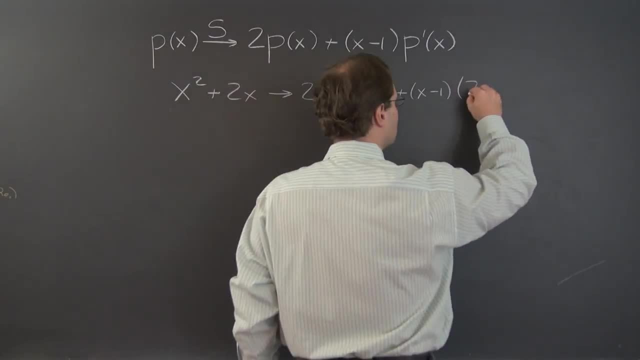 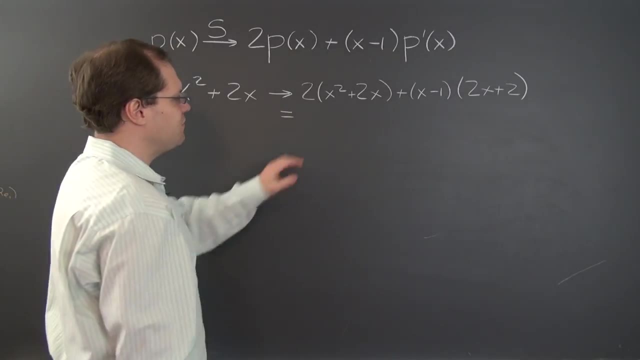 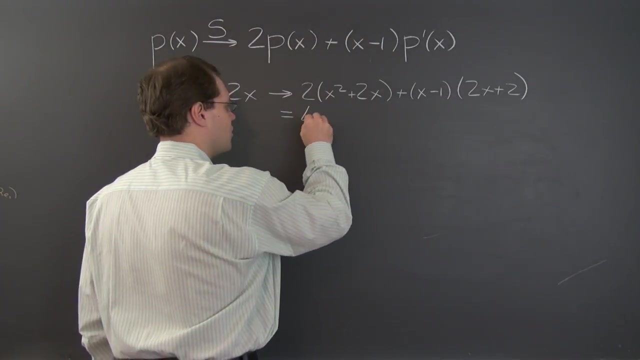 Which is 2x plus 2.. 2x plus 2.. Alright, and now let's simplify the result. and we find collecting the powers, so x2x squared plus 2x squared, so it's 4x squared.